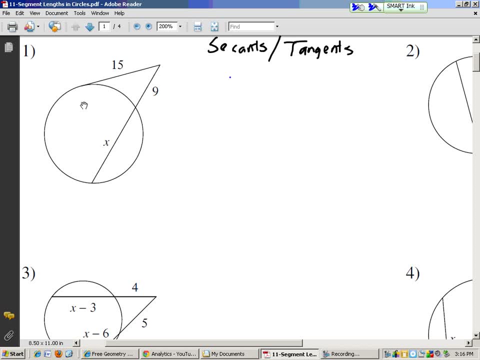 So if they're secants and tangents intersecting outside the circle, we're going to use this formula of ow, ow, Outside times whole equals outside times whole, So outside times, whole. So as we look at this, let's look at the secant. for starting, This is the secant. 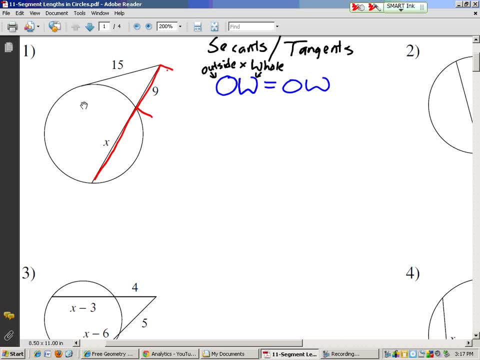 And the nine is the exterior product. This is the outside portion of that secant. We're going to call that the outside portion, So this is going to be nine times the whole portion. So what's the whole portion of the secant? 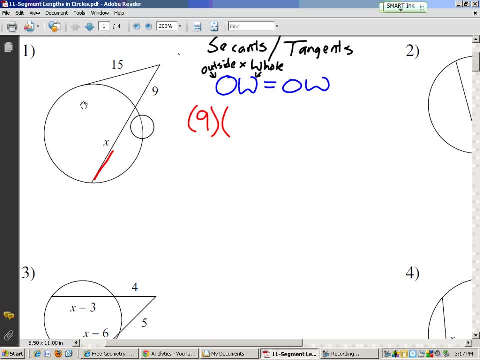 Of course. yeah, I definitely think that my video processor's got a little more nick and handle Doing recording and everything. Give me a second, I'll see if I can get that to all go away. All right, so the whole portion of this is going to be the nine. 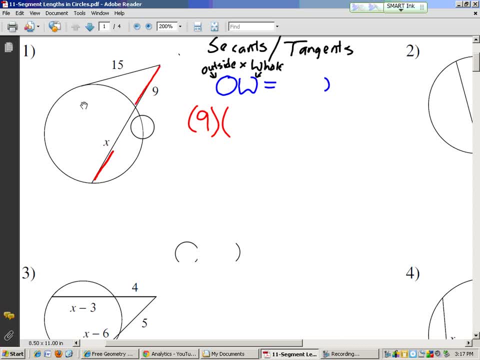 All right, so the whole portion of this is going to be the nine. All right, so the whole portion of this is going to be the nine plus. So the outside times whole is going to be nine plus. So the outside times whole is going to be nine plus. 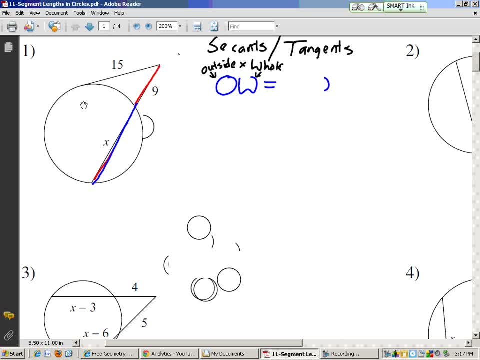 Let's see if I can get that to come back. Yeah, I think she's gone forever. There we go, perfect. So nine plus x- Now the outside of the tangent- this is going to be your tangent in green, because it only hits once- is equal to 15,. 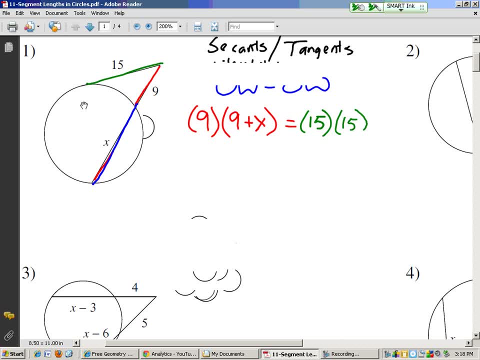 15, and the whole is also equal to 15.. All right, so now let's multiply this and I'm going to distribute here and I'm going to get. 81 plus 9x equals 225.. Subtracting 81 from both sides. 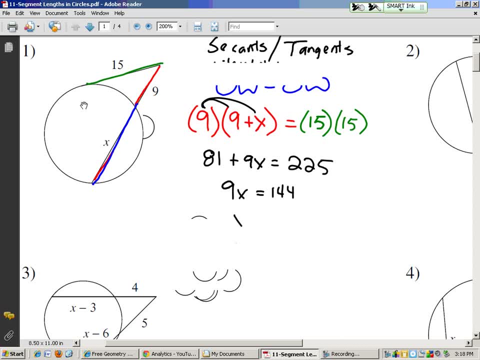 I'm going to get 9x equals 144.. Dividing by 9,, I'm going to get x equals 16, and I'm done These. don't take that much work Later. I mean everything that's new, everything that is. 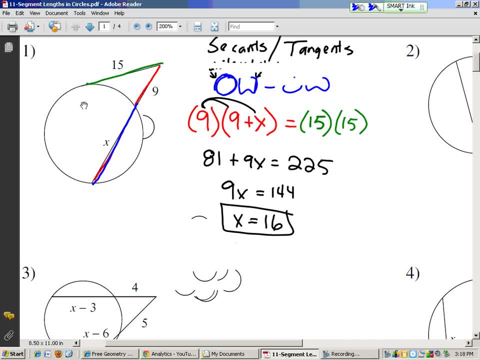 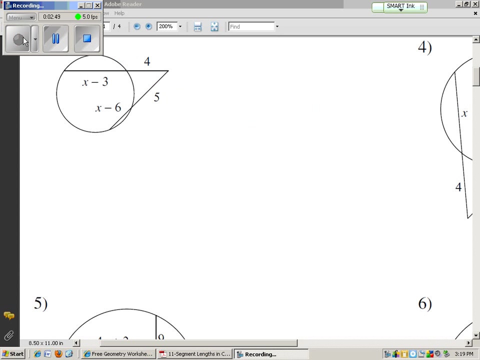 geometry is located inside this formula: al, equals al, so al, al, and identifying what these shapes are: secants and tangents. All of this from here down, that's all just algebra, and you guys have already had that class. All right, we're going to move on. The next problem I'm going to do is 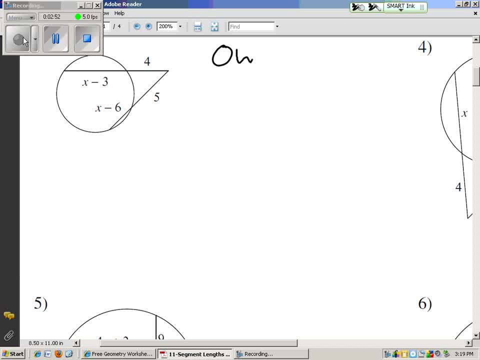 number three. I'm going to do number three. I'm going to do number three. I'm going to do number number three. I'm going to do number three. I'm going to do number three, I'm going to do number three, and so we're going to once again, because these are both secants, I'm going to use al al. 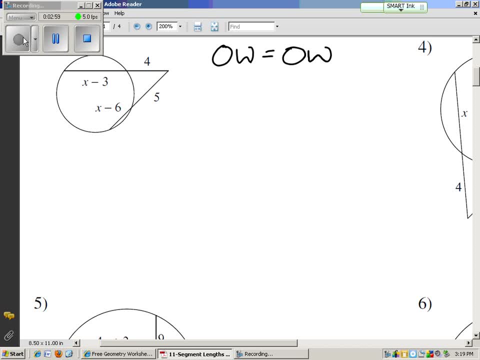 so outside times whole equals outside times whole. So the outside of the upper secant is equal to four and the whole upper secant is going to be four plus x minus three. So that's going to be four plus x minus three, and the outside of the lower secant- this part here- is going to be equal. 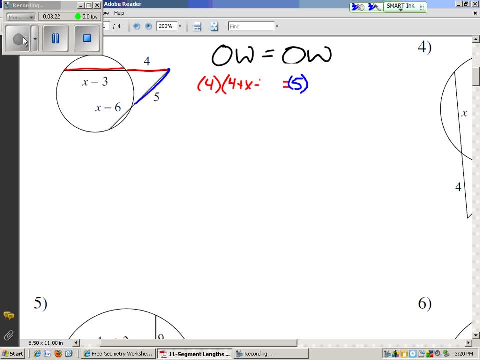 to five, and then the whole lower secant is going to be five, plus the other section of this, which is x minus six. I know that half of this erased, but I believe I've got four and a minus three here, right. So that's going to be four times x plus one when I put those two together. 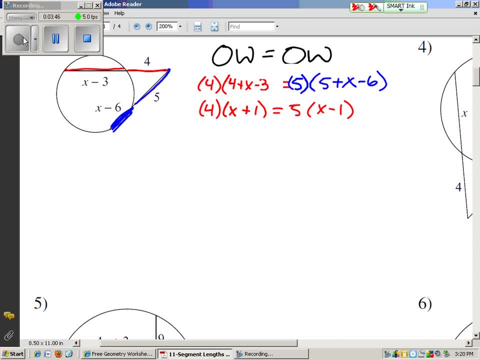 and this is going to be five times x minus one. when I put those together and then as I distribute, I'm going to get four x plus four equals five x minus five. and I'm going to subtract four x from both sides and add five to both sides, I'm going to get nine equals x. 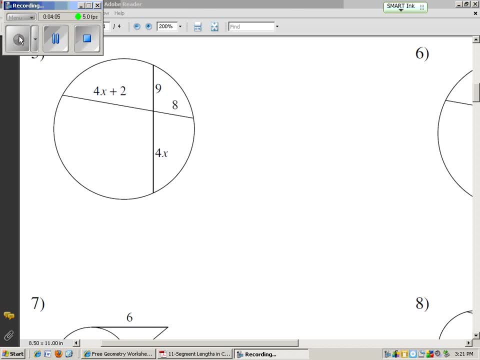 Easy, cheesy Number five. So, on number five, I'm going to use a different formula now, because this is two chords, Two chords crossing inside of a circle. These two cords cross right here and they have portions. So I want to look at the 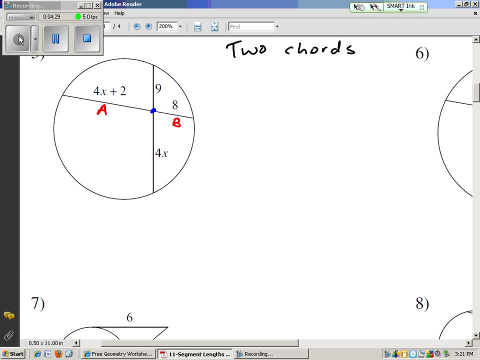 portions of one side. so I'll call these A and B, and the portions of the other side. let's call this C and D, and those are going to be multiplied together to equal each other. So what I'm looking for is A times B equals C times D. So let's go through and plug that in. Well, A is going to be. 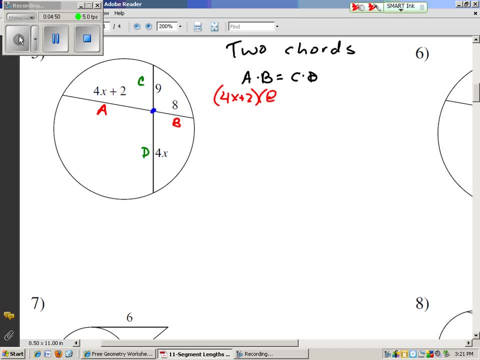 4x plus 2,, B is going to be 8,, C is going to be 9, and D is going to be 4x. Multiplying this out, I can distribute the 8 to the 4x and the 2, and I get that 32x plus 16 equals 36x. 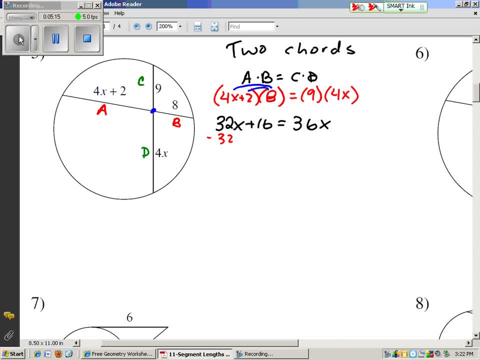 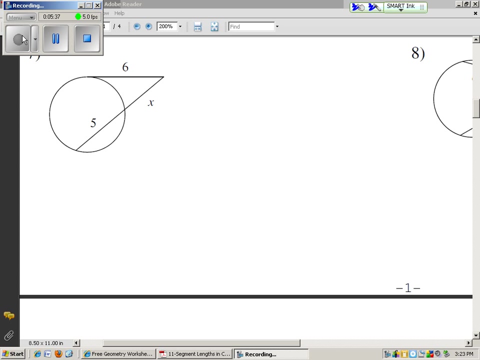 I can subtract the 32x from both sides and I get that 32x plus 16 equals 36x And I get 16 equals 4x. divide by 4, x equals 14.. Done, So number 7 appears to be a pretty simple problem. It looks about as easy as number 4, say: 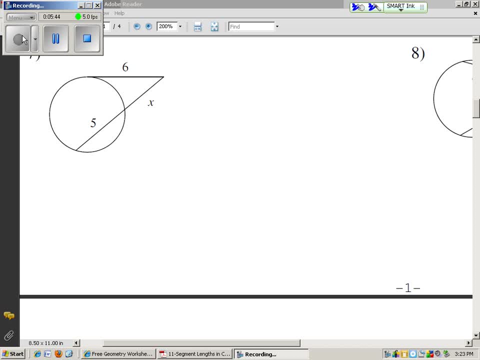 I wouldn't see much difference in it except for the location of the x, which is what's going to make the difference. So if we go back to our LL, L equals L outside times. whole equals outside times, whole. So let's start with the tangent, because it's easy. I get 36, right, That's going to be. 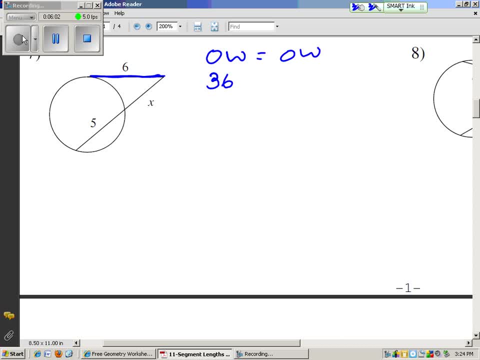 outside is 6,, the whole thing is 6.. So multiply those together and I get 36.. Why waste time, right? So the other one, though, outside is x and the whole is x plus 5.. So I got to add those together. 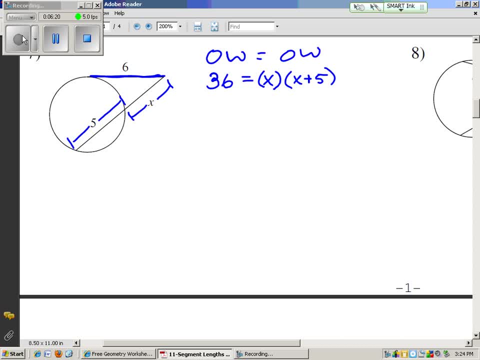 x plus 5. 5.. Now we start to see where this is going to go wrong. When I distribute this, I'm going to get 36 equals x squared plus 5x. Now stop copying me at this point and let me show you, because I know. 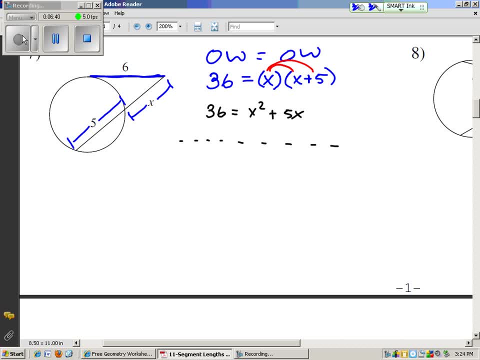 a lot of you are saying: well, Mr Conaway, there's a square, You take the square root, so let's try that idea out. I guess what you mean by that is: let's subtract 5x from both sides and let's see. 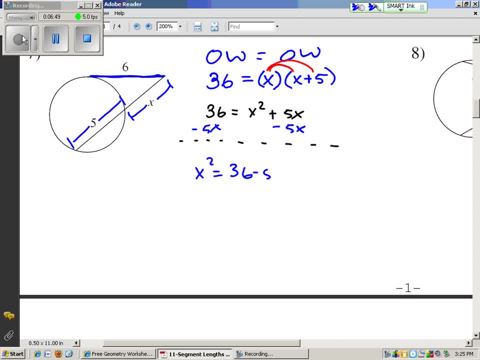 if I can get x squared, equals 36 minus 5x, And then if I square root both sides, I'm going to get x equals the root of- well, positive or negative root of 36 minus 5x. Now the question is: is x? 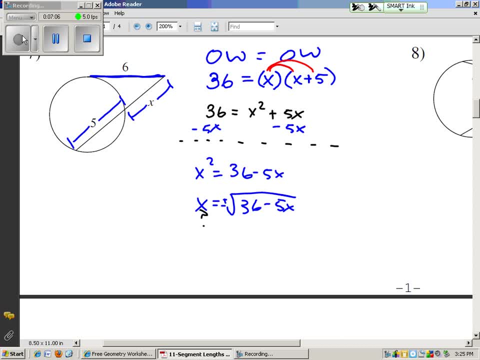 alone. Can I define x in terms of another x? Can I say that an object that is circular is shaped like a circle? Can I say: circles are round, Round things are circular. No, because I'm defining something in terms of itself. I cannot use something to define itself And therefore this is not really solved. 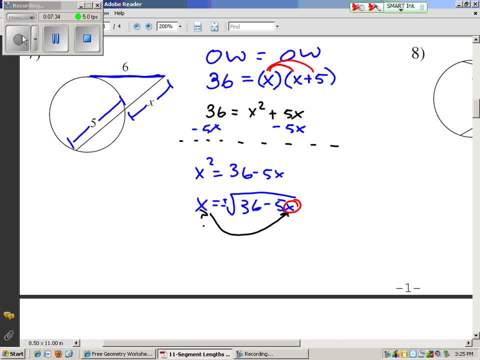 if another x is on the other side. I have not actually solved it, So I need to not think this way And let's go back And look at how to do this the right way. So let's solve this by making a trinomial. I'm going 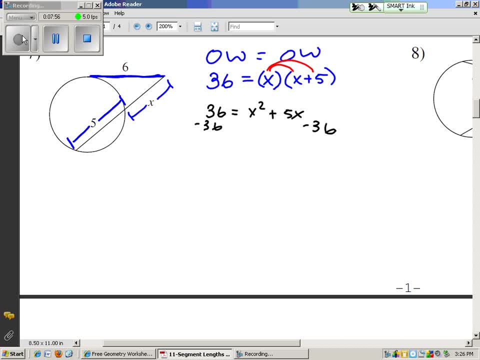 to subtract 36 from both sides, And I'm also going to do a big flip-flop. We can always switch sides of an equation, because equations are symmetric, They go both ways. So x squared plus 5x minus the 36 that we had right here, equals. well, these two are going to go away and be zero. So now I have 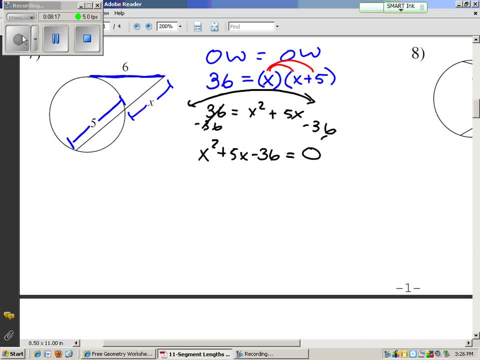 a nice trinomial And we learned back in Algebra 1 that to deal with a trinomial, we're going to factor that trinomial. So we're going to say: well, x and x obviously go here, because x times x equals x. 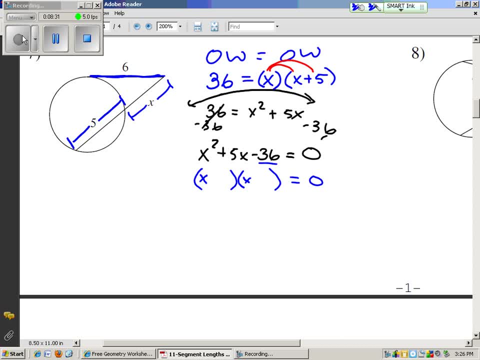 squared. But now I need things that multiply to give me a negative 36.. But when I combine them using addition or subtraction, they come up with a 5. So what multiplies to be 36?? Well, 1 and 36,. 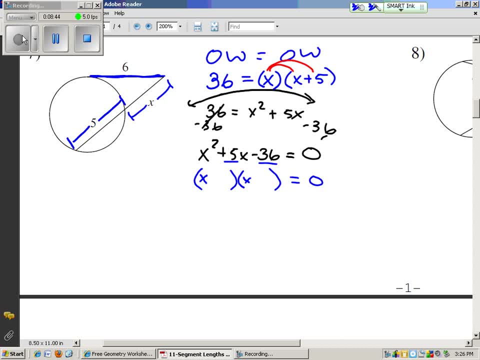 2 and 18,, 3 and 12,, 4 and 9,, 6 and 6.. Which of those could I Add or subtract to be 5.. Yeah, So 4 and 9,, as my class is trying to tell me here, So 4 and 9.. But 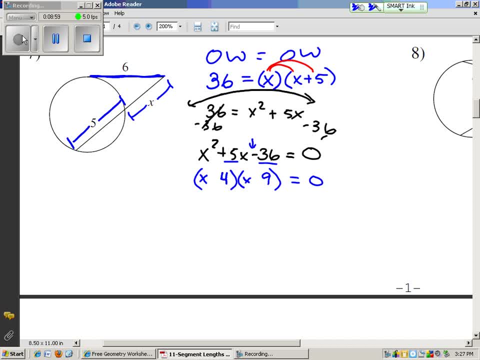 in order to get a negative on that 36,, one of these has to be negative. So yeah, if we and my class once again says negative 4,, positive 9,, then when I add these I take a positive 9x and. 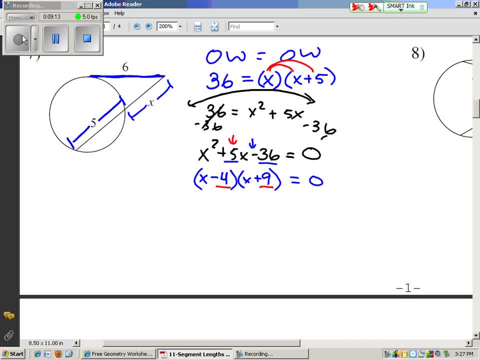 a negative 4x, and together they do make a positive 5x. So yes, I'm good I've got this done. But just in case I can check it out: x times x is x squared, x times 9 is 9x Minus 4 times x. 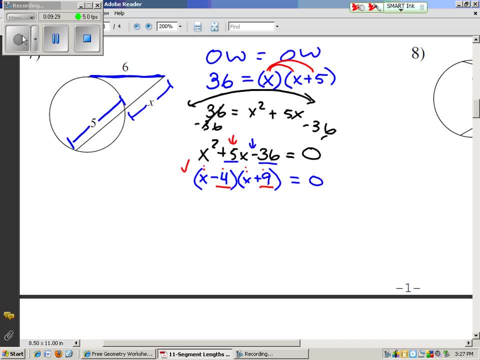 is minus 4x. So 9x minus 4x is 5x. We got that. And then minus 4 times 9 is minus 36.. We've got that. So this definitely works. Now for the next step, and some of your teachers may not explain.